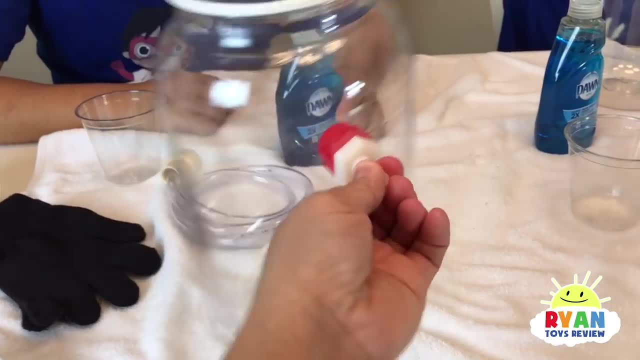 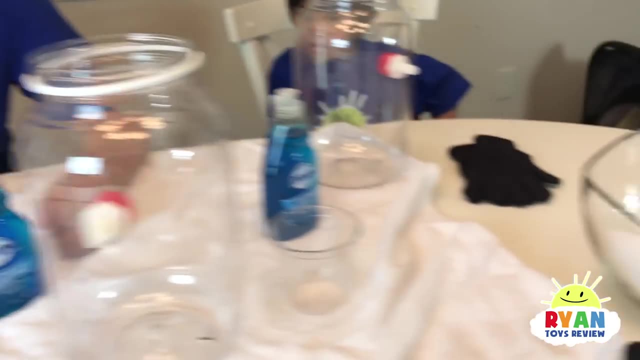 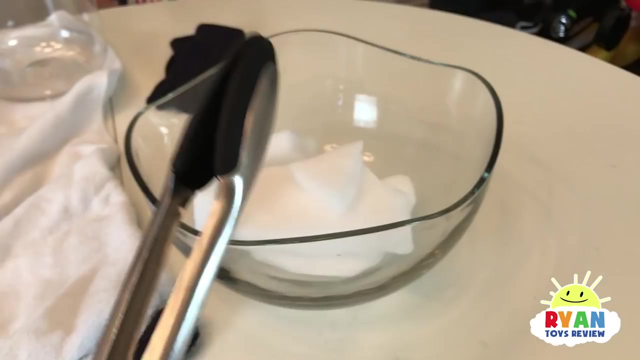 containers here. You can make your own, but we bought ours, And then you need this hose to attach, And then you need some Dawn soap And then the dry ice, And then never touch the ice with your hands. So we're going to use these tongs here. So what we have so far, this is warm. 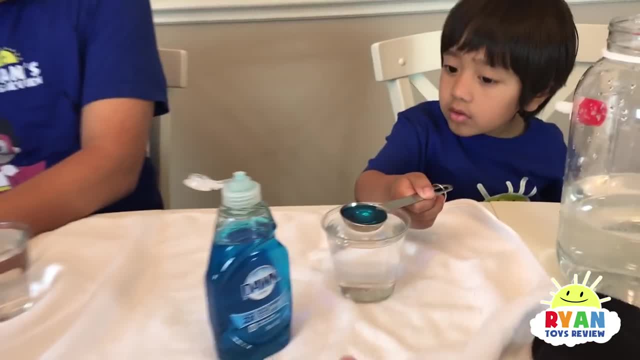 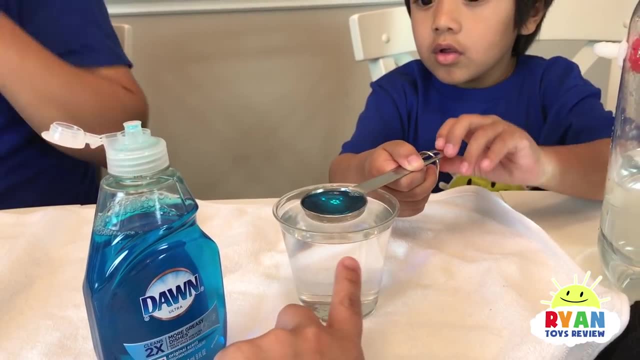 water in the big bubble generator container And this is just regular distilled water. And here we have Dawn soap. So Ryan's going to put two tablespoons. We're going to put one tablespoon of Dawn soap into this smaller cup. Drop it. 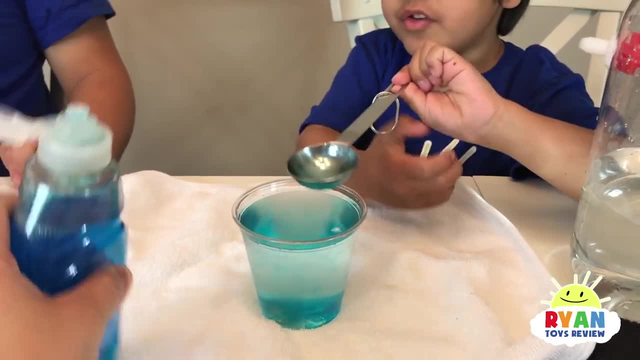 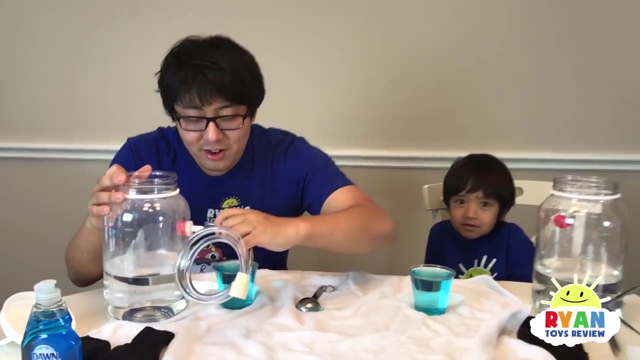 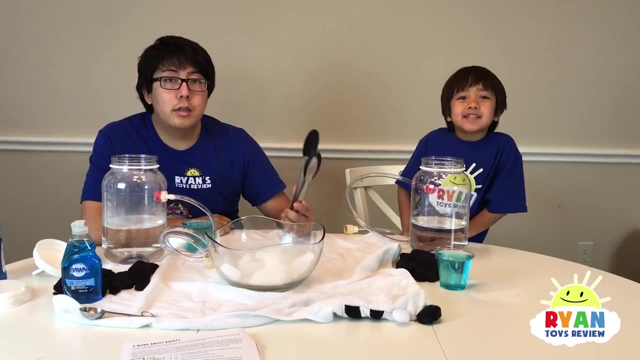 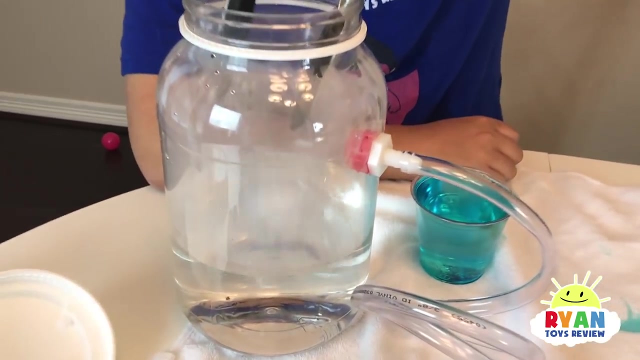 There you go. One, And we need one more. So attach the tube to the bubble generator. Push it really hard. Next, let's put the dry ice inside. Yeah, So here it is. Never touch the dry ice with your hands And don't eat it or put it in your mouth. 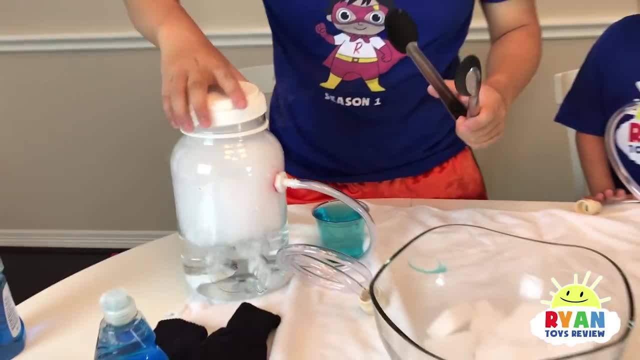 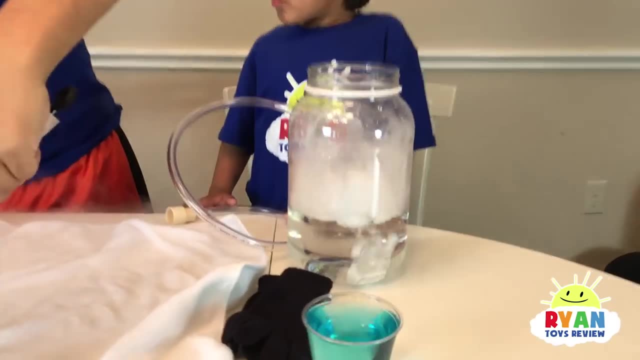 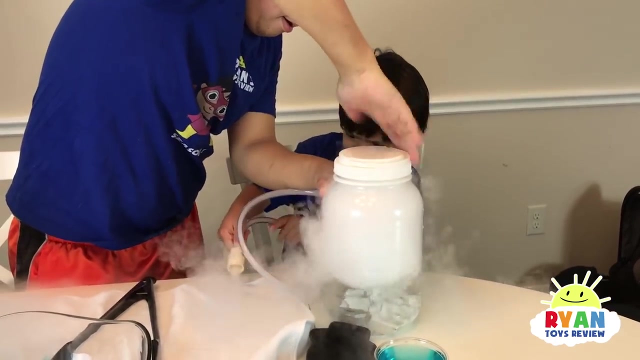 You want more? Yeah, Here you go. Come on, Whoa Caught it. Whoa, Can I do it to yours, Ryan? Yeah, Do it to yours. Do it to Ryan's one. Close the cap, Whoa. 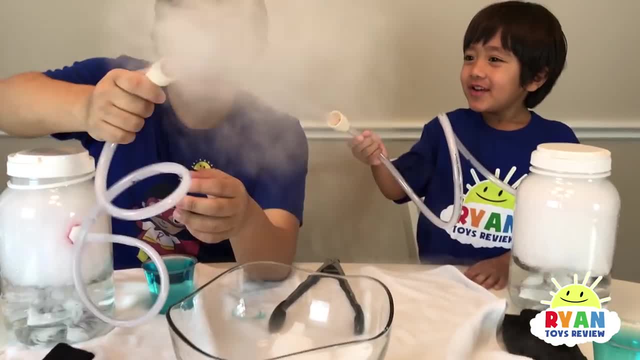 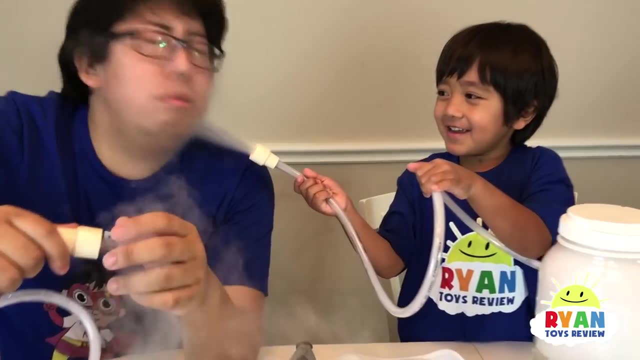 Open my mouth, I'm in trouble. Ha, Look A box coming out. Ooh, Is it cold? No, Oh, yeah, It's a little bit cold. It's good for you. Oh, Oh, Ooh, It's cold, Whoa. 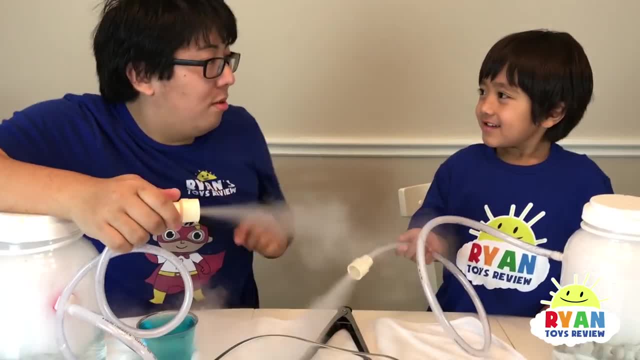 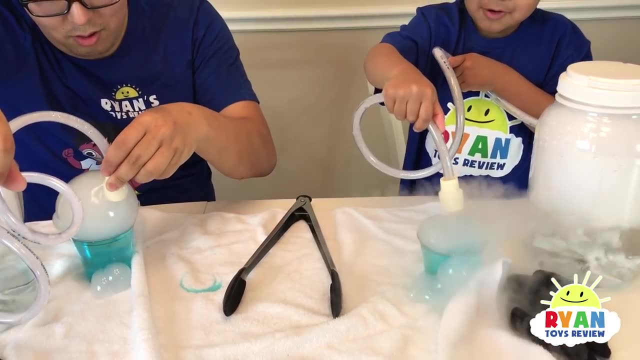 That's funny. Ooh, That's so cool. Yeah, that is funny. Oh, Is it cold? No, I'm just kidding. Now let's dip it in. Whoa, Whoa Dip, Like, dip it in and take it out right away. 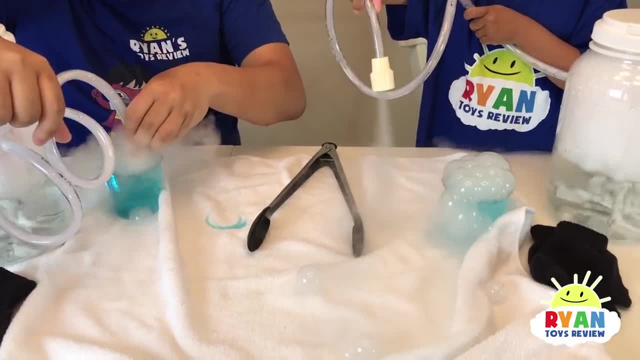 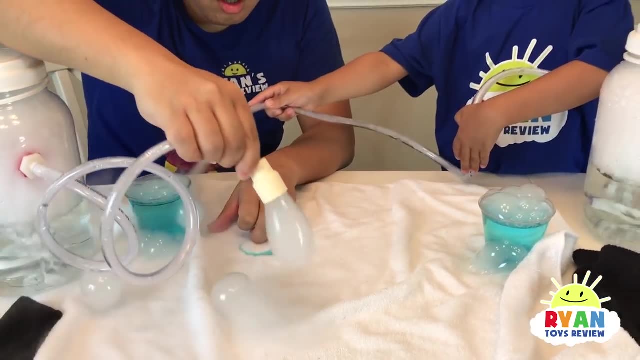 Oh, okay, Yeah, Oh, Boo bubble. Oh, Ryan got his first boo bubble. Look at that. Look at the boo bubble. Whoa, You got to do it fast, or something You have to hold. Oh, I'm blowing. I'm blowing it so it's popping. 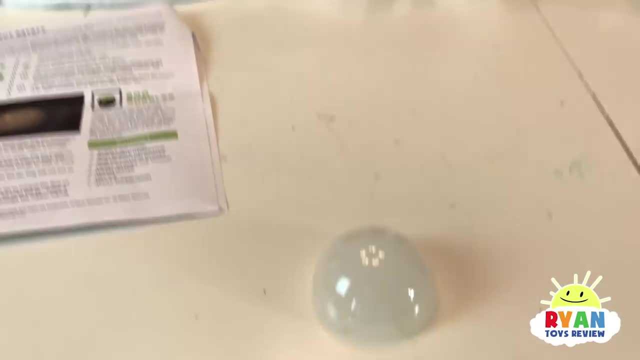 Whoa. Look at the boo bubble. Whoa, Whoa, It just balls a boing, boing, boing. Yeah, That's so cool. Let me touch the boo bubble. You can touch it, Ryan. Now you can touch it. 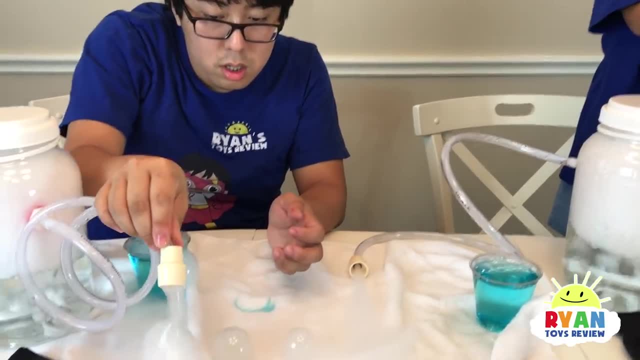 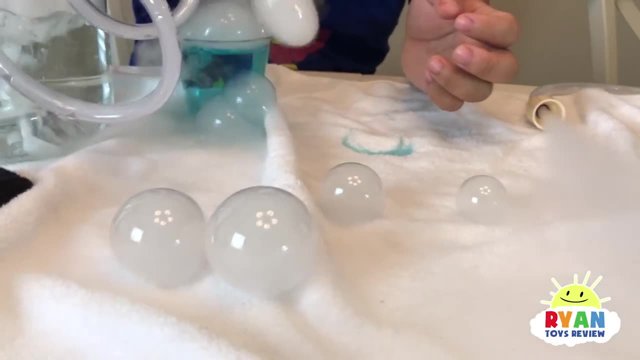 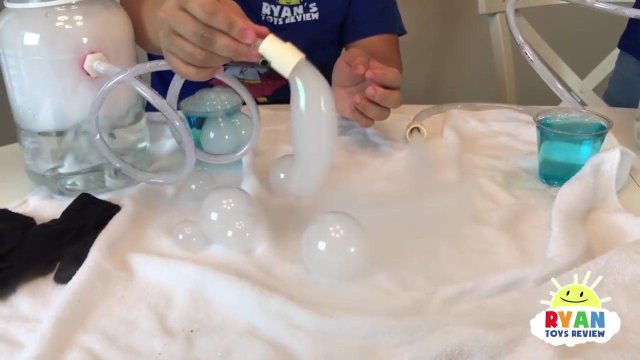 It's just like bubbles: You can pop it. I don't want to pop it, I want to just hold it. Whoa, Look at that. It's kind of a little bit tricky. Is this hard for kids? No, It's just hard to get used to it. 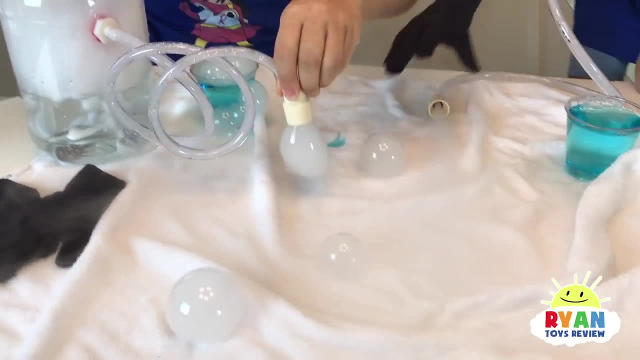 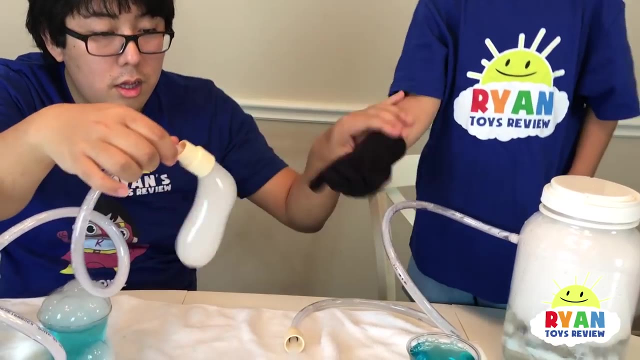 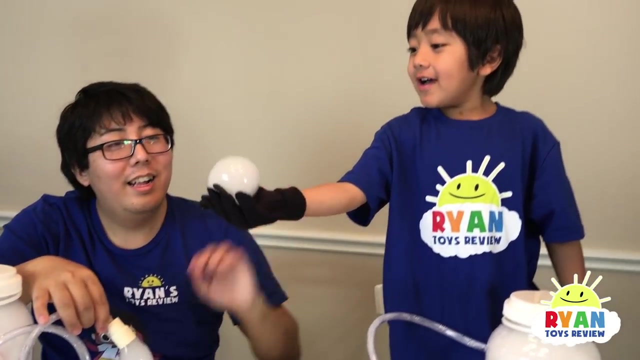 Wow, That's so cool. Daddy, can you make a boo bubble? Put it on Ryan's hand? Okay, Put the glove on. Oh Hard, huh. There it is. Wow, That's cool, That's funny, That's fun. 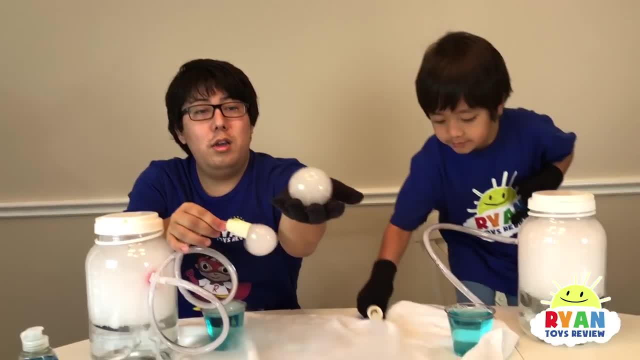 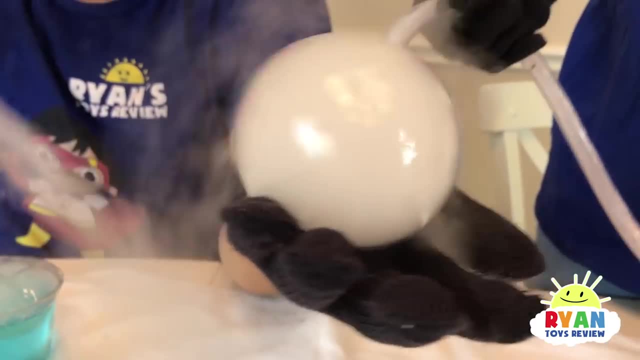 Whoa, Whoa, Whoa. Look at that. Oh Oh, My first boo bubble, Your first baby boo bubble. Wow, Look at Daddy's bubble. Boing, boing, boing, boing, boing, boing. 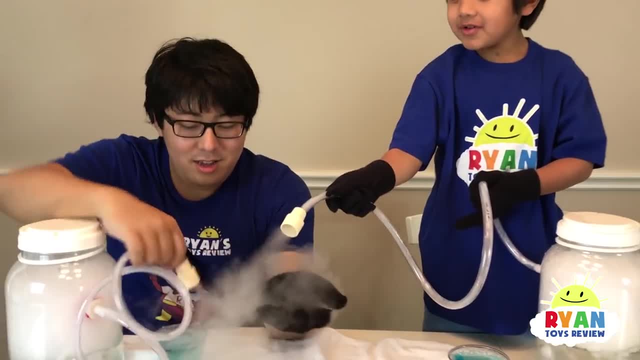 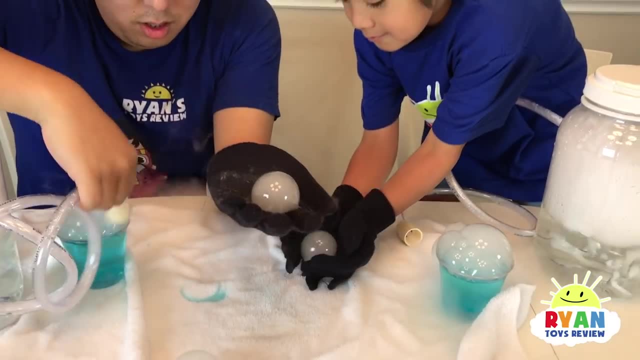 Whoa Hey, Hey, It needs a lot of air to pop. Oh, Ryan's boo bubble. Look at that. Good job, Ryan. Whoa, Ryan picked it up. Yeah, Good job. Oh great, So you're going to do it. 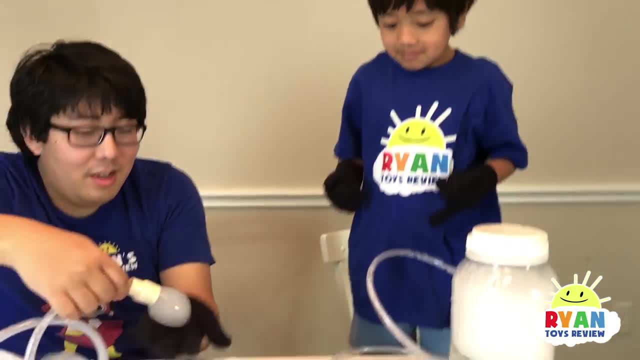 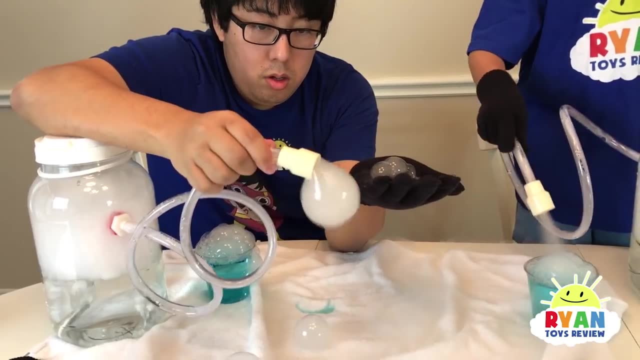 Okay, So you're going to do it. Okay, Yeah, It's usually regular bubble busts when they touch anything. So the bubble pops when they touch oil or dirt, But because it's on cotton, it doesn't pop. Look at that. 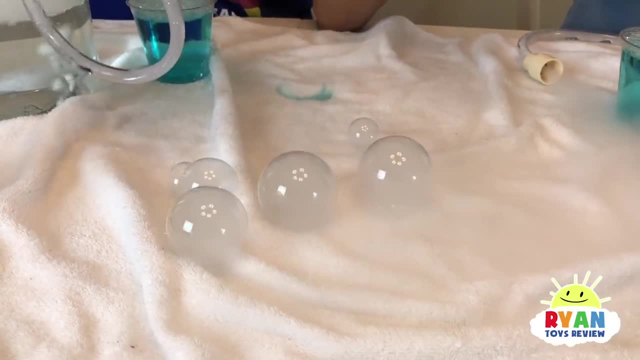 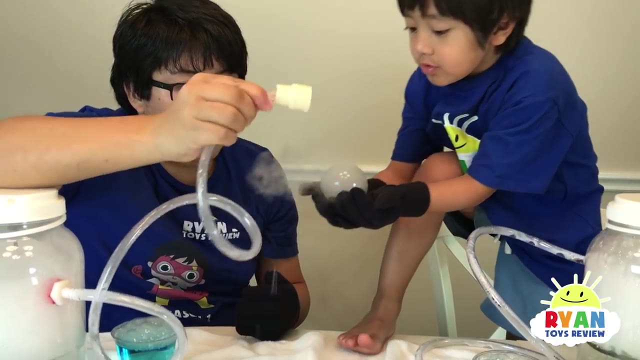 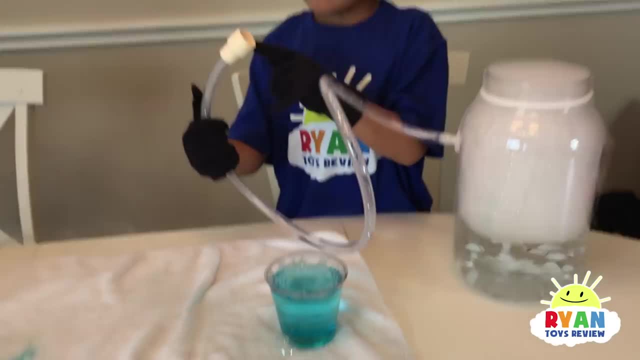 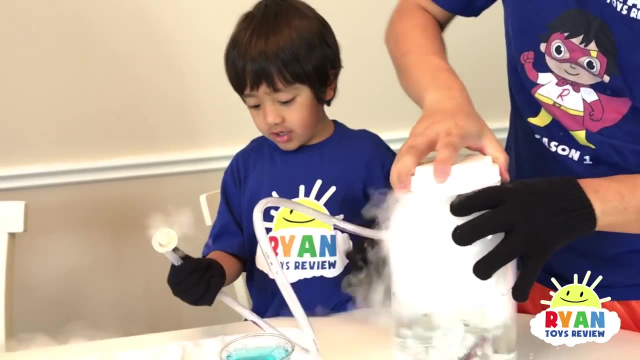 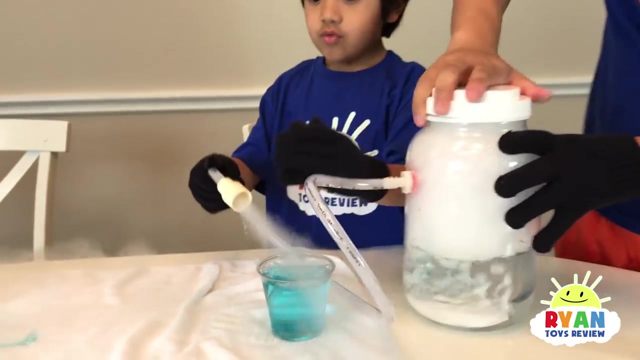 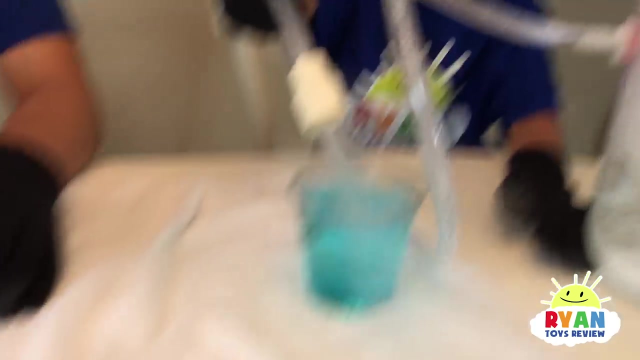 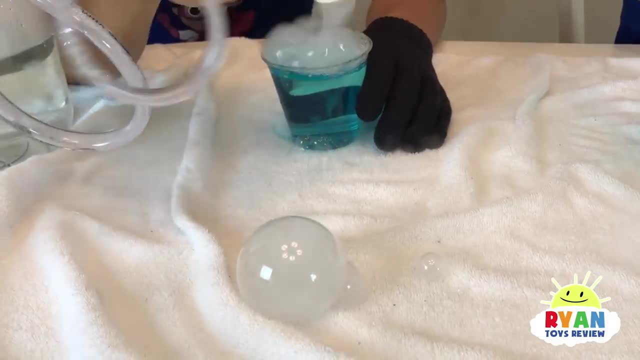 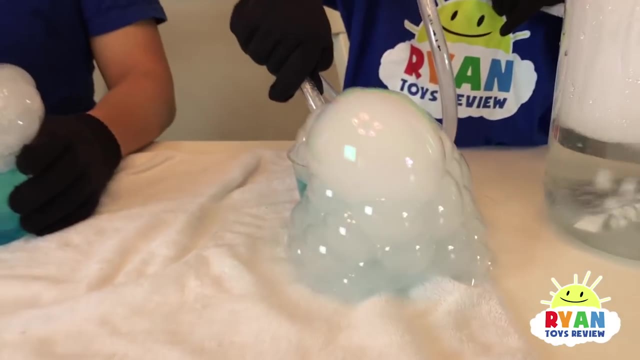 See, connect and make a big boob bubble. Connect them. Whoa, Ryan, Daddy, Oh my gosh, Oh, a giant boob bubble. Whoa, Oh, a giant boob bubble, Daddy, Oh my gosh. 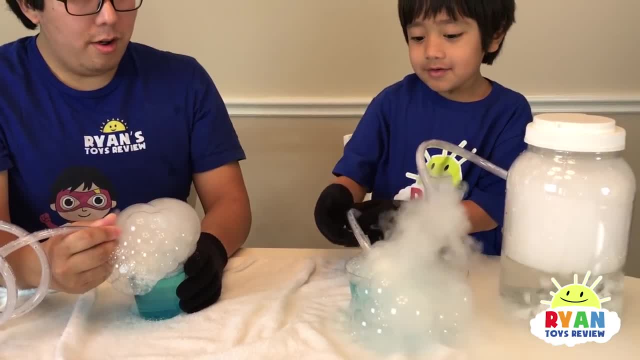 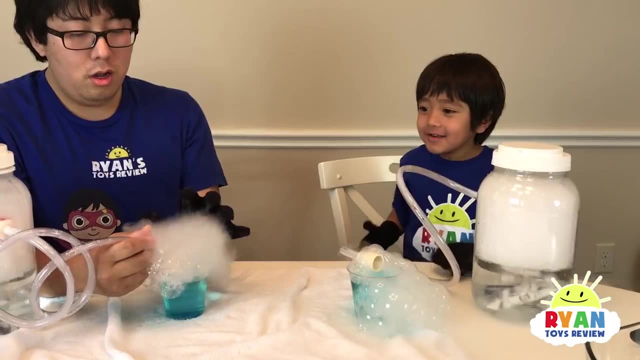 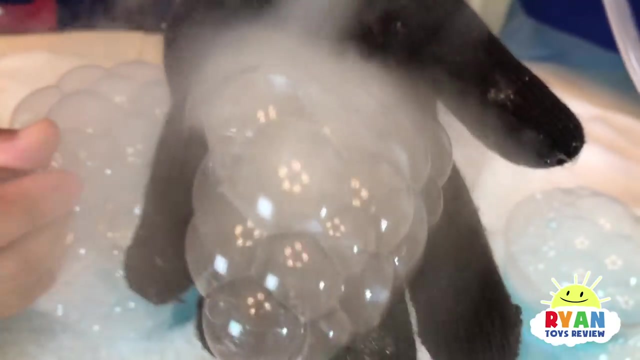 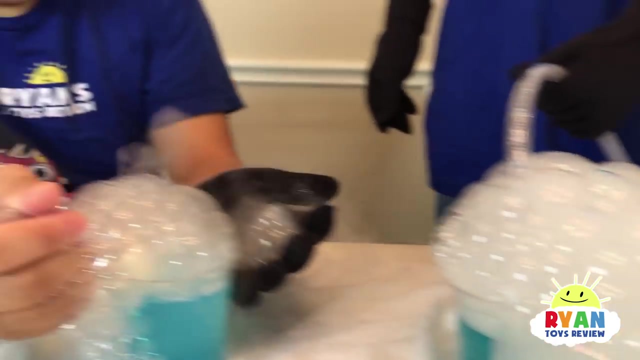 Bubble explosion- Whoa, good job, Ryan. Oh, my gosh. Whoa, Oh, I can touch it. Whoa, giant boob bubbles. Funny. Whoa, Yeah, cold. Wow, I'm amazed, Daddy, your bucket isn't filled. 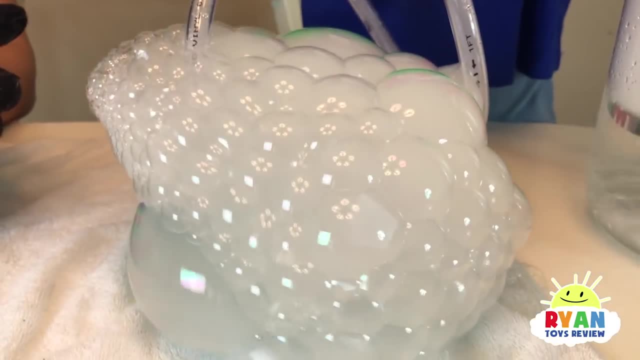 My bucket's filled. Yeah, it's a race, Ryan's winning. Daddy, Whoa, Whoa, I can't even see the cup. Yeah, Where are you? cup Whoa still coming out. Pop, pop, pop, pop pop. 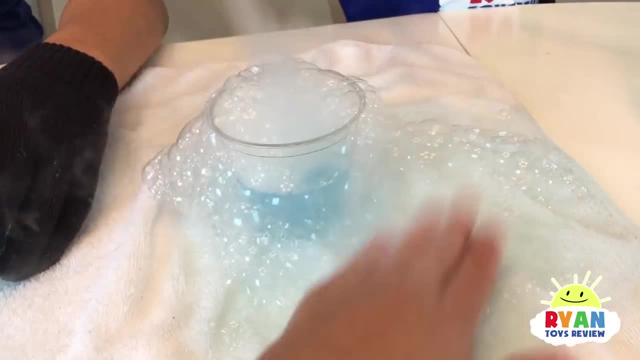 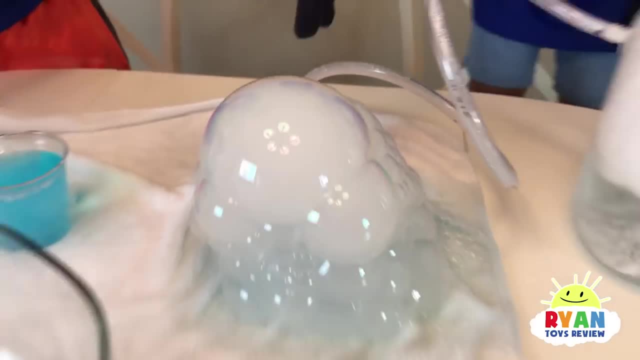 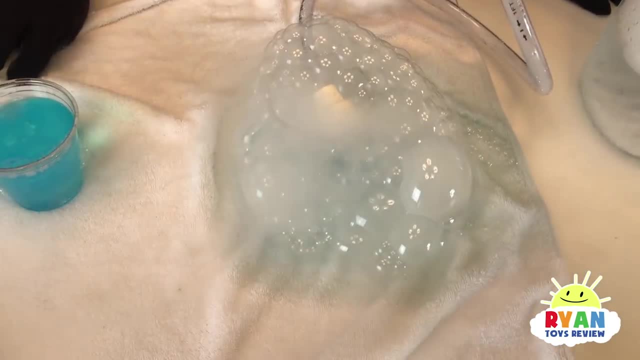 Wow, That's the biggest food bubble I ever seen. Whoa, I saw the pots. Yeah, that was cool. We're going to put some toys in for a swim. Ooh, PJ Masks. Hi boys, By the Maze. 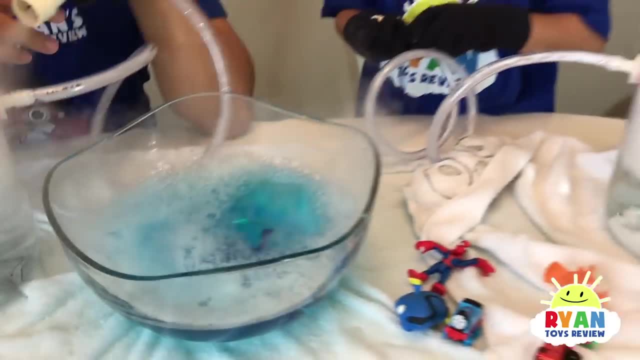 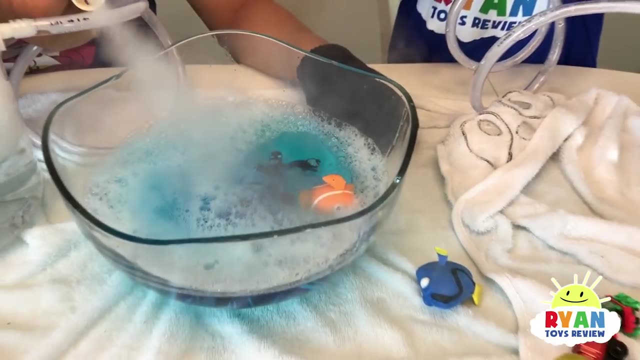 Heidi, Nemo, Thomas Wait, Nemo's swimming. Everybody's not swimming, That's true. Dory Dory, Dory, Percy, Percy, Percy, Dory, Dory, Dory, Dory Dory. 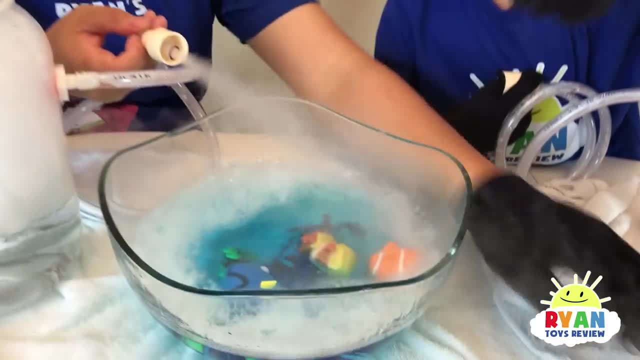 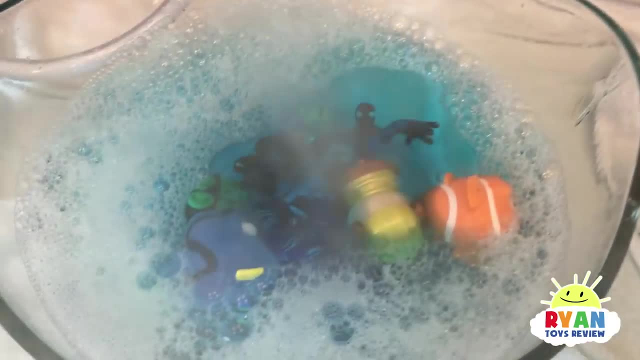 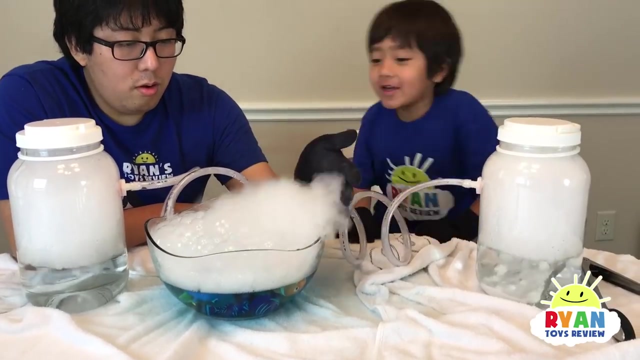 Let's put the whole thing in Rubble. I think only Masha will swim. James, James Minion- I don't think it swims. Minion arms developеры. Let's put the whole thing in There it goes.